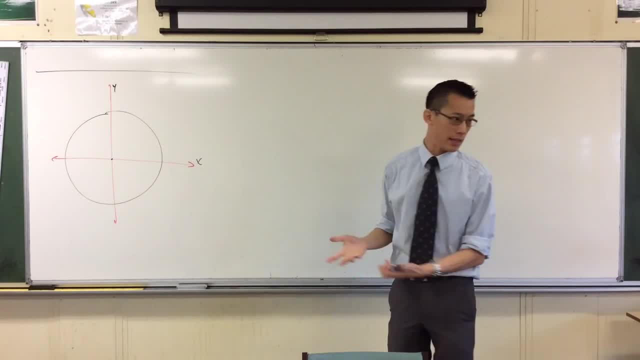 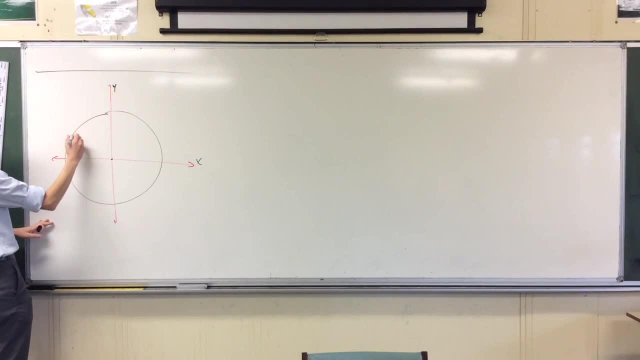 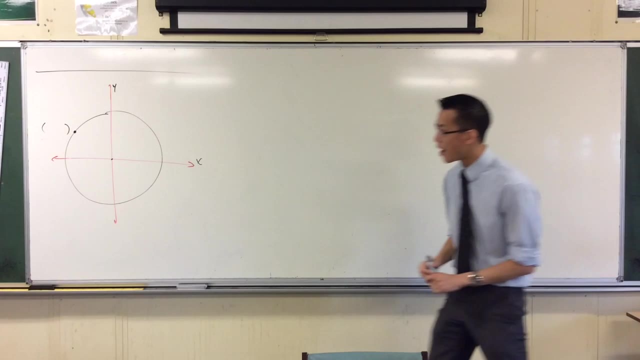 I know how to define any point, not only in this space, but any point on this circle, right. So, for instance, I could pick a point over, say I'd estimate about there, and because I'm very good with my unit circle, I've been using it for a long time. 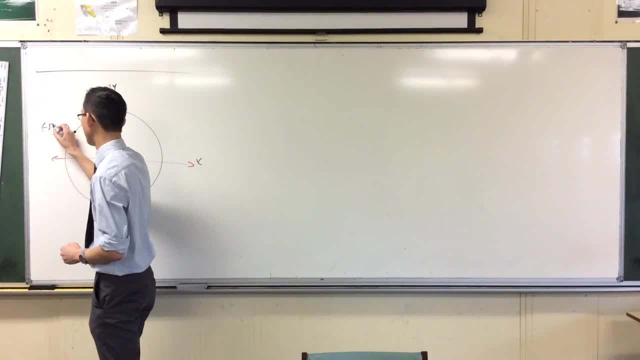 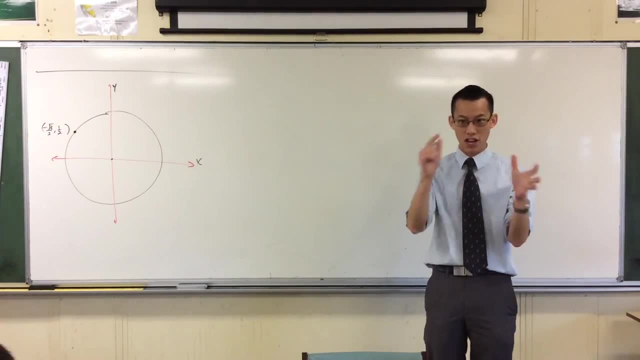 I know that its coordinates are roughly well- not roughly exactly- minus root 3 onto a half. okay, Now I can plot that around, I can go around, I can check on graphic software etc. I'll get values like that. 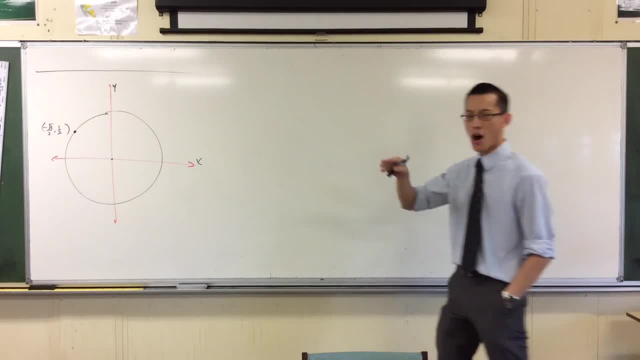 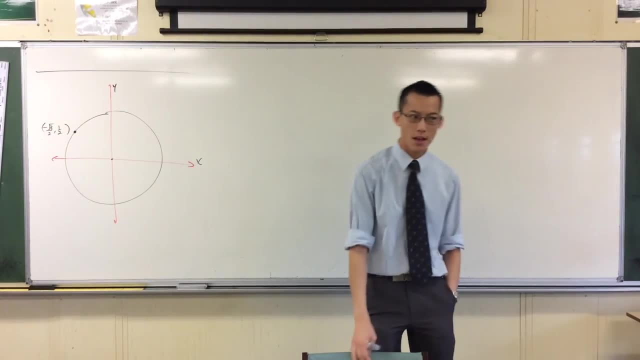 In other words, I'm defining a point by horizontal. good morning, horizontal and vertical displacement. We were used to calling these Cartesian coordinates, But we learned that there was another way of defining points on this circle, Another pair of values that I could use to uniquely define any point where I am right. 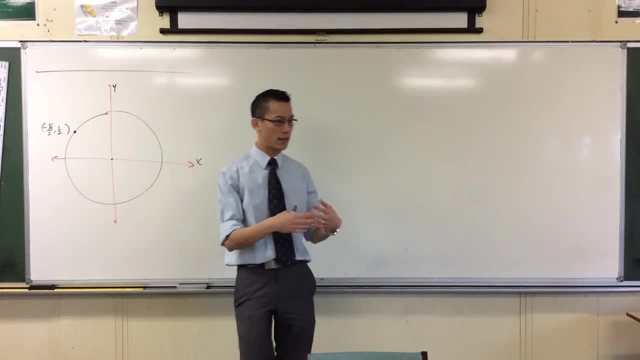 Instead of going horizontal, vertical, instead of going Cartesian right, What was my other pair of values I could use? Okay, so I could use. actually, on the unit circle, I only need one value If I say, alright, there's a point over here. 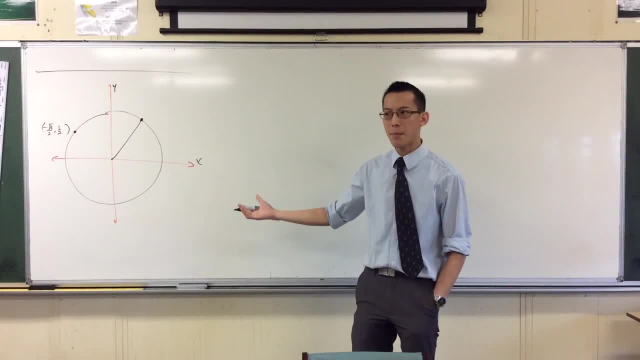 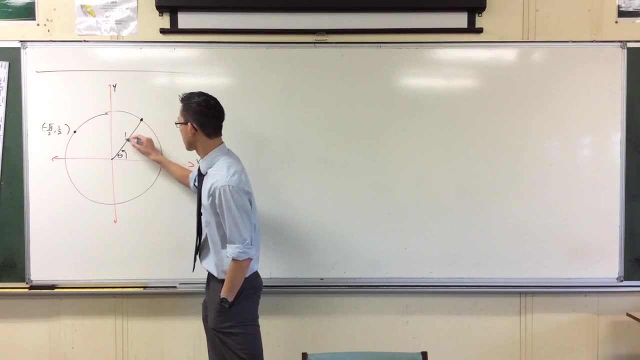 There's a point over here. okay, To know where I am on the circle, all I really need is the angle, and I've already told you the other piece, which is the radius right. Once you know the angle and the radius, I can tell you anywhere you are right. 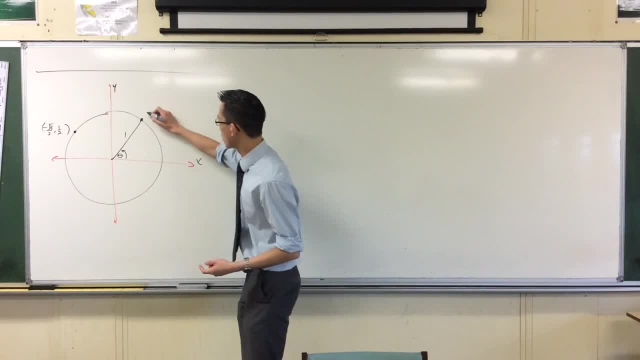 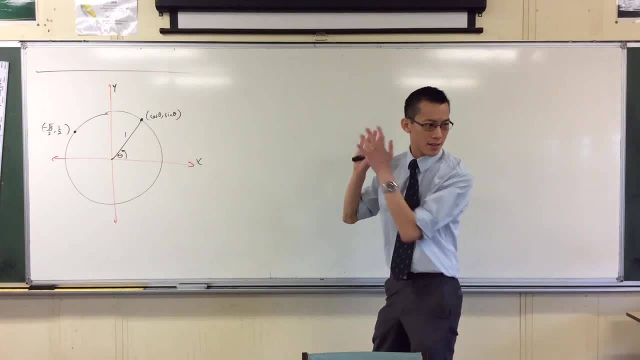 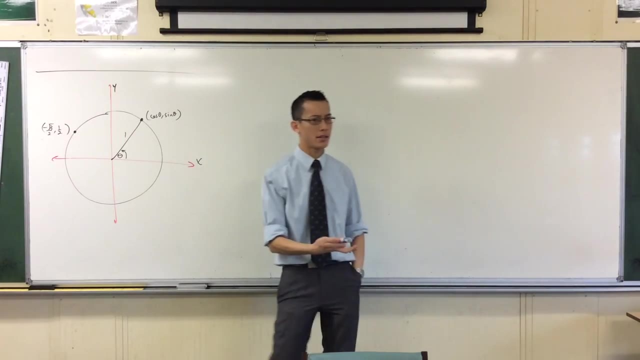 So these are not Cartesian coordinates, they're also called Palmer coordinates. So we've got cos theta sine theta here, right? So this is the first time you need a parameter, and then we've worked into parametrics. Now, the reason why I've drawn this comparison is because when we were trying to look at complex arithmetic- right? 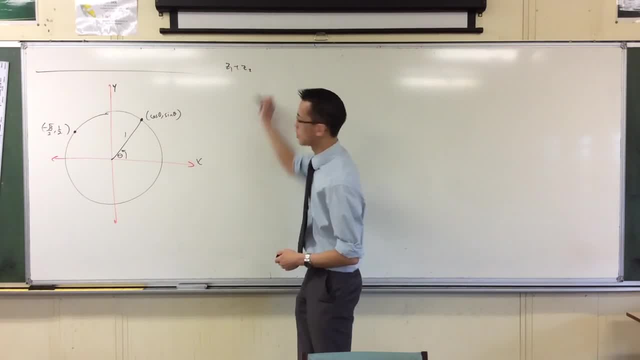 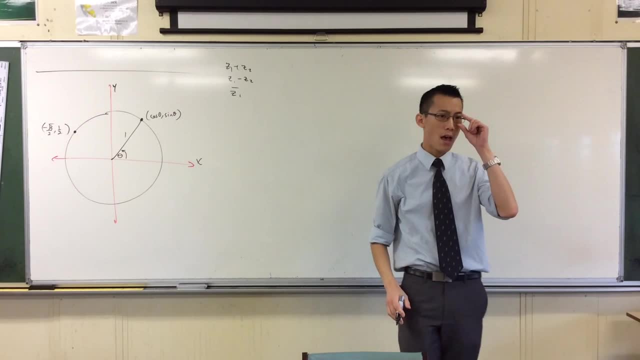 We talked about what happens when you add numbers. we talked about what happens when you subtract, when you take the conjugate, etc. right, And then, when we got to multiplication, we noticed that the geometric meaning of multiplying complex numbers has to do with a certain number. 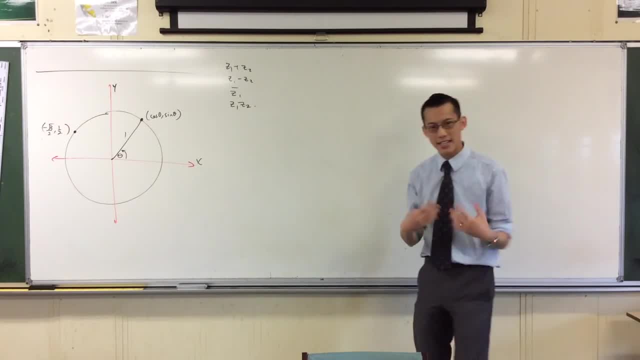 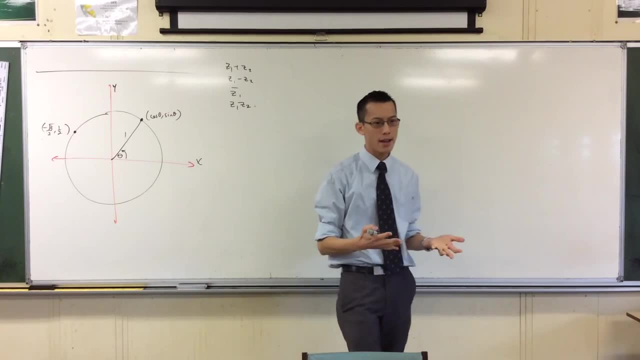 We noticed that the geometric meaning of multiplying complex numbers has to do with a certain number, has to do with a certain number, you with rotation. Do you remember that, In a sense, complex numbers have rotation baked into their structure, in the same way that integers, numbers with a sign, have direction? 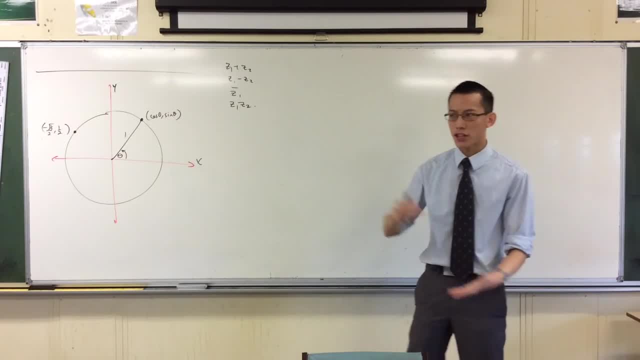 like back and forth baked into their structure. You can just add positive and negative numbers together and you can just go left and right or up and down however you please. It's like part of the DNA of the number And part of the DNA of complex numbers is rotation. 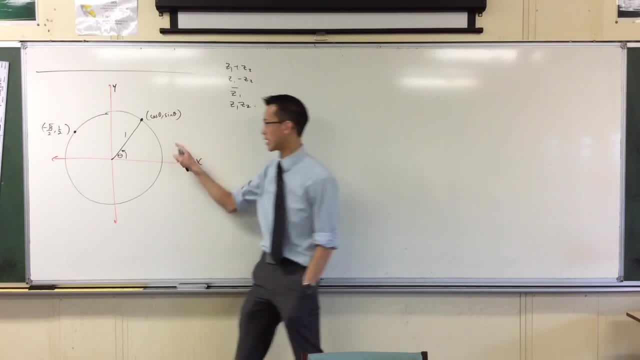 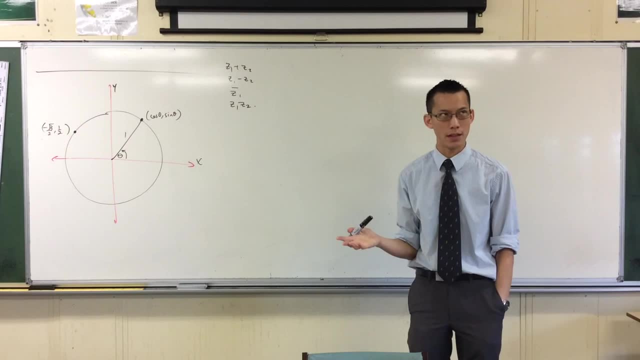 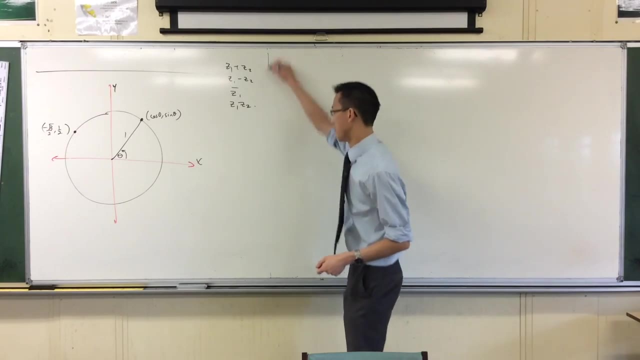 So, being that I can define numbers like points on the inner circle, like this, I can define complex numbers- which in the last few lessons we've been talking about complex numbers- as points. I can do them in exactly the same way. So, under all of this, this is my review. 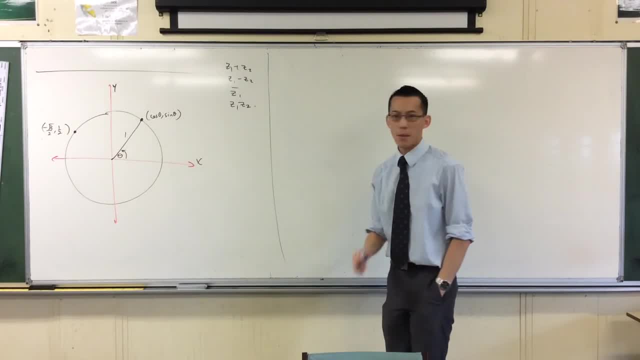 and trying to build a bridge into this new idea, give me a little subheading And, by the way, this is still not the proper heading. we'll get there in a second, A little subheading, which is representations of complex numbers. 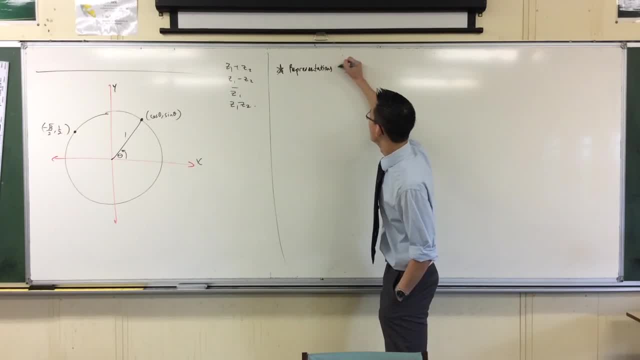 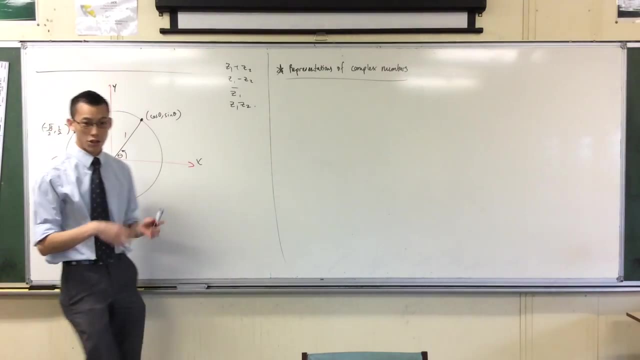 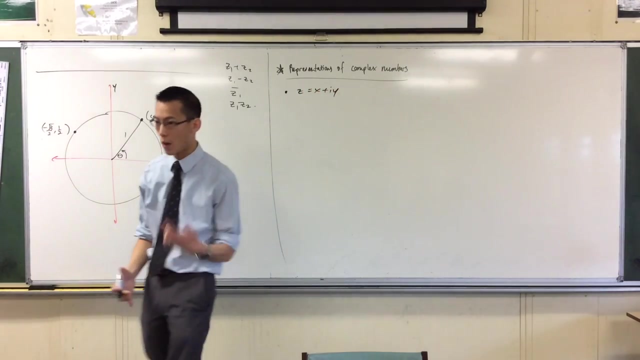 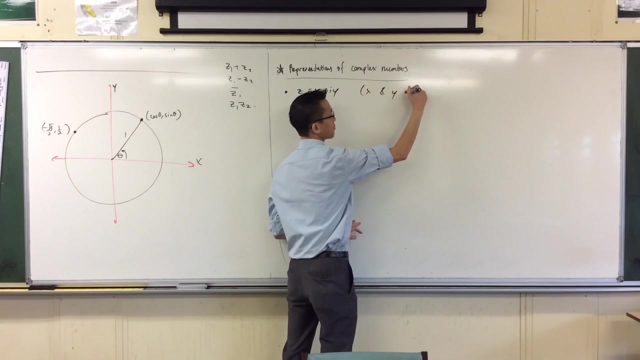 So the first one again, which corresponds to this guy here, and the one that you already know, is to say: z equals x plus iy. that's one representation of a complex number. Now, what are x and what are y? Right? X and y are they're about go this way? there's much. 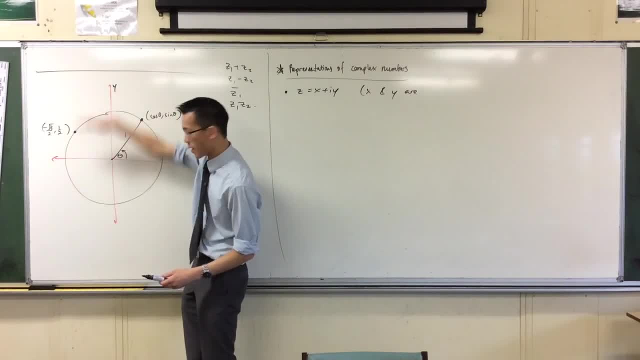 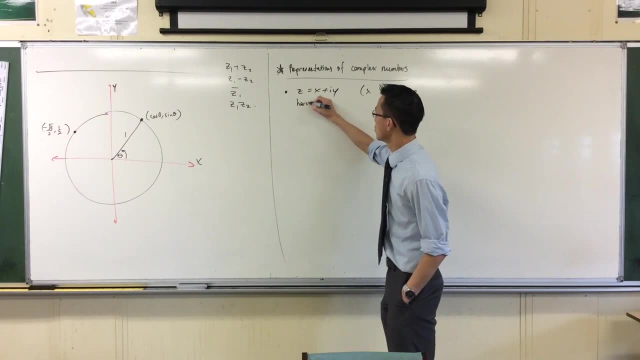 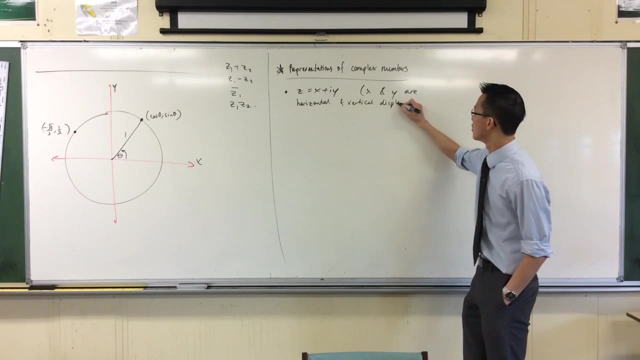 go this way. this much. They're about that horizontal or vertical division. So x and y are horizontal and vertical displacement. How far do you want me to go In this direction? How far do you want me to go In this direction? 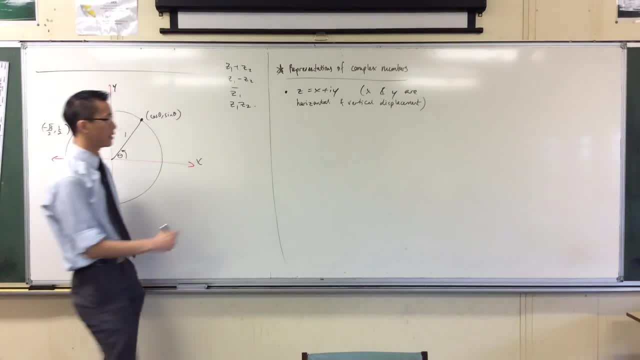 In this direction. Once you tell me those two things, I'll be fine, But there's another way of stating this, and it's on this form here. I still need two numbers because I'm still in a two-dimensional space, but my two numbers are quite different. 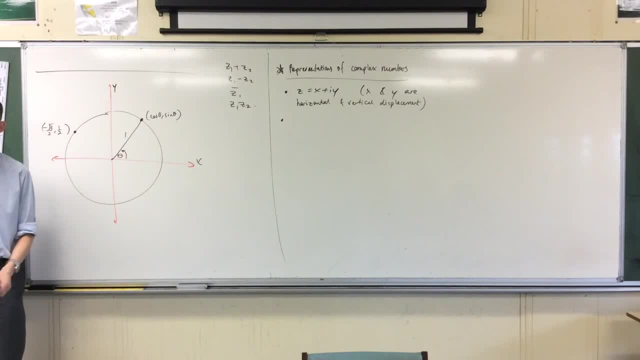 They don't correspond to horizontal and vertical displacement. They correspond to number one, an angle, this angle here, and number two. how far do I go in that direction? So the angle tells you which way would you like me to face. 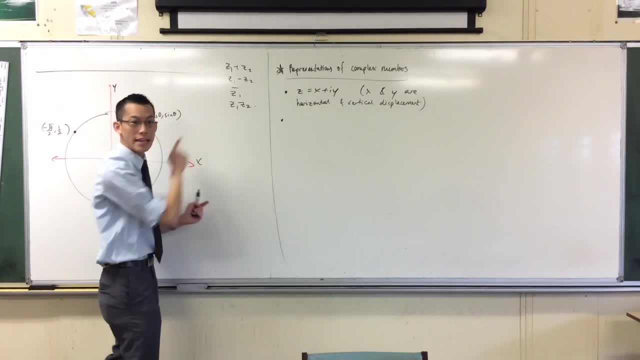 and then this number here tells you how far should I go in that direction. So instead of z equals x plus iy, I'm going to say z equals. Now I'm going to borrow this same result that we established from the unit circle. 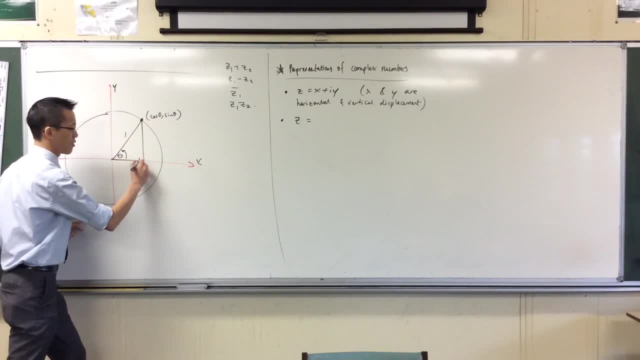 The cos, because if I make a right-angled triangle here, you can see the reason why cos theta is this horizontal component. Okay, Because in this triangle cos theta is adjacent on hypotenuse Cos theta, And up in here I've got the vertical part being sine theta. 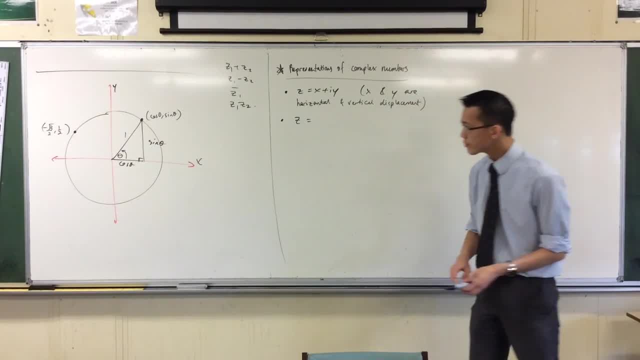 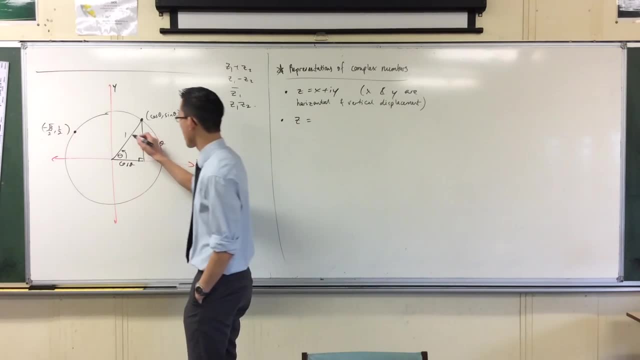 All right, let's extend it just a little bit. Extend it just a little bit. If I am no longer on the unit circle, right, because the unit circle is just one circle. if I have a circle of radius r, how does that change things? 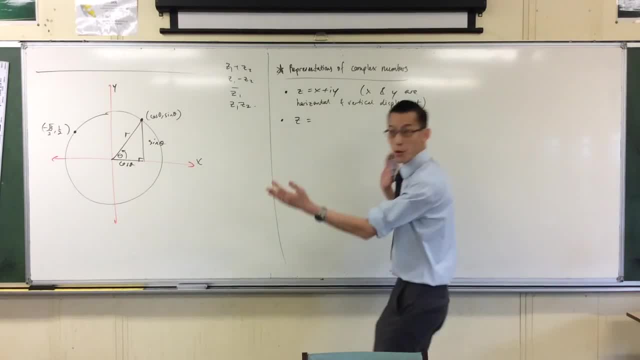 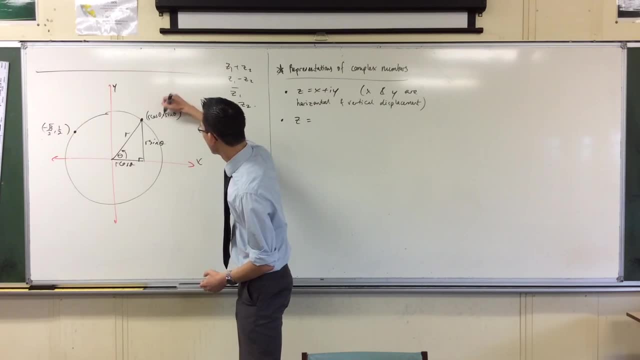 How does that change my coordinates? Okay, good, I'm going to be further away, so I won't just be cos theta, I will be r cos theta, I'll be r sine theta. So I've got my coordinates changing like so. 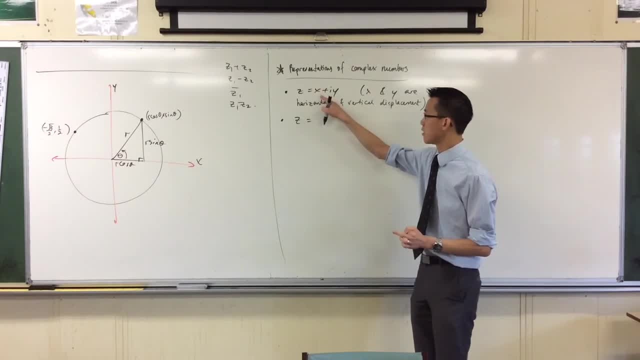 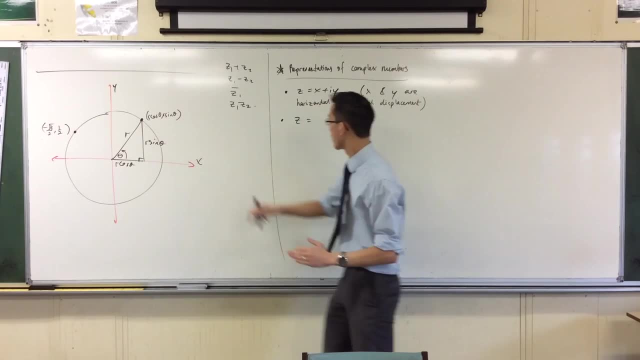 Now, therefore, if I write down x plus iy in terms, of this is x my horizontal part and this is y my vertical part, right? I would say: well, the x part is r cos theta. That's the real part. 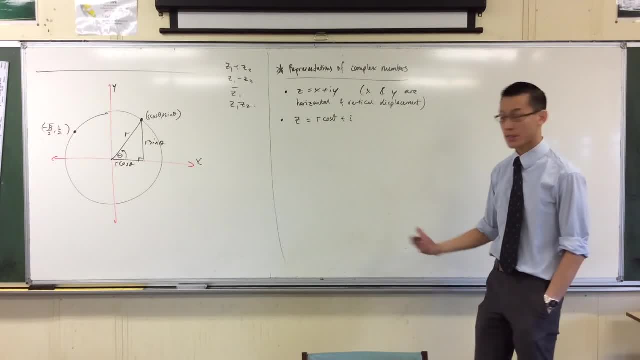 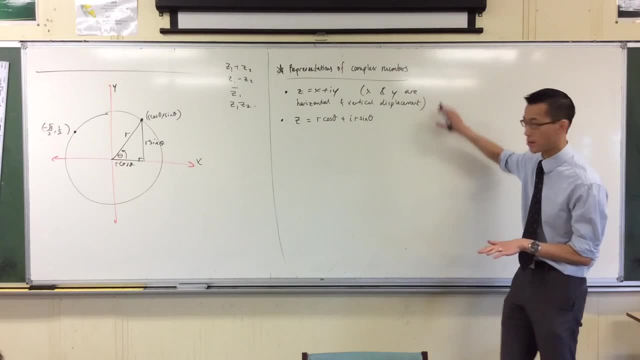 And I've got i times r sine theta, And that is the imaginary part. okay, Now I'll just tidy this up. before I make a summary here, I'll take my r out the front, because it's a common factor, And then you'll see this: 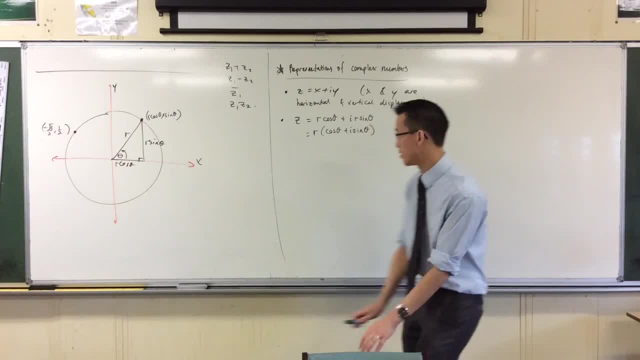 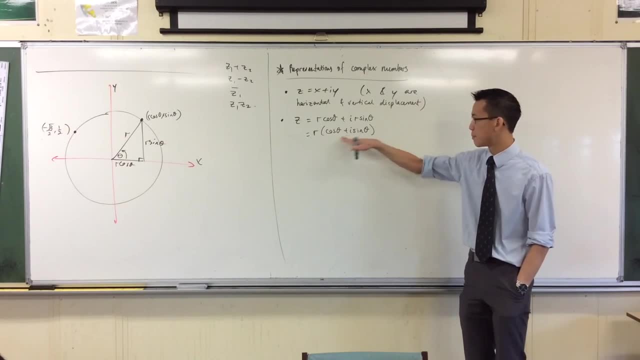 Okay, Now I'm going to write down one extra line after this, which I'm not a huge fan of, but you need to recognize it. okay, Can you see? you're going to get cos theta plus i sine theta, which corresponds to well. 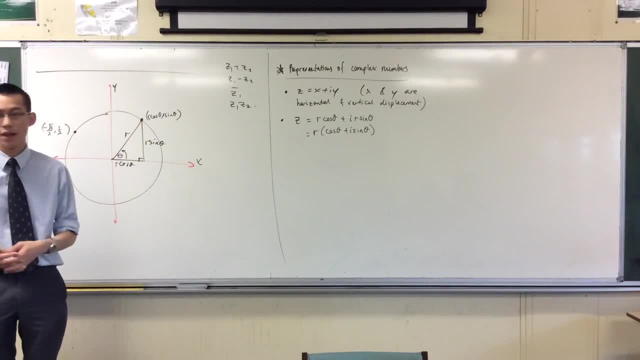 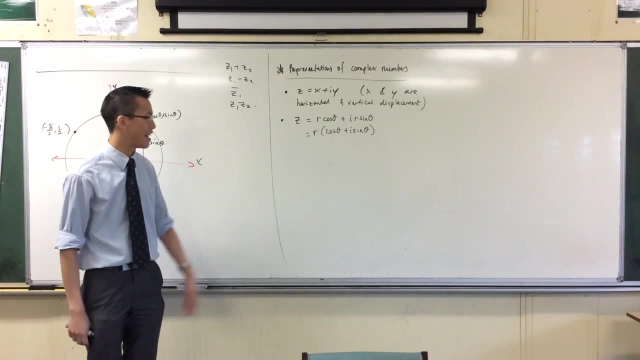 just where am I horizontally, Where am I vertically? But I'm thinking in terms of an angle. now, okay, Because you'll get cos, and then you'll get this i sine part over and over again. right, And it gets a bit tiresome. 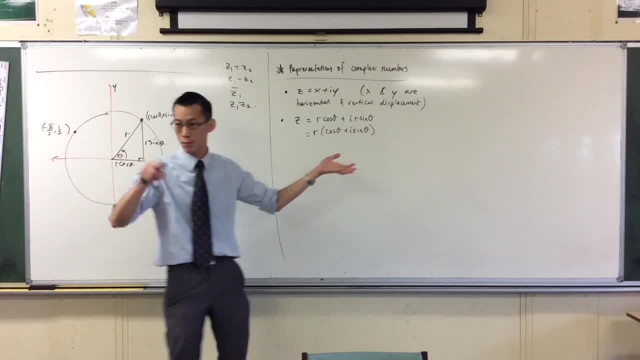 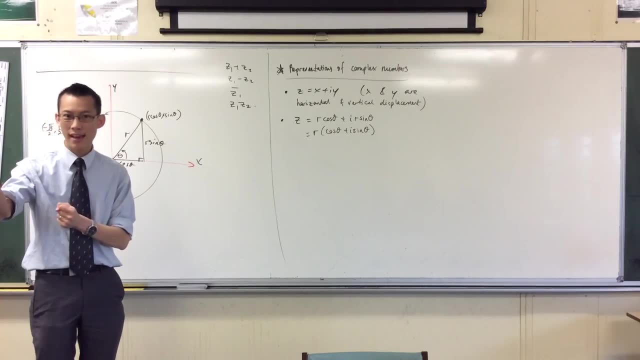 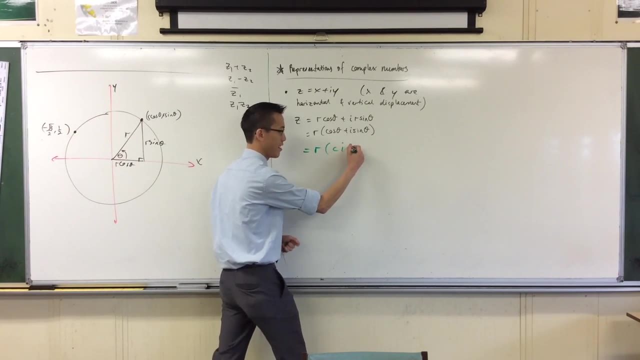 Like you'll always have the same theta in both places, because it has to be to represent a point in two-dimensional space. Some textbooks will contract the cos and the i sine theta into c for cos, i for imaginary s for sine, And then the angle is going to be the same. 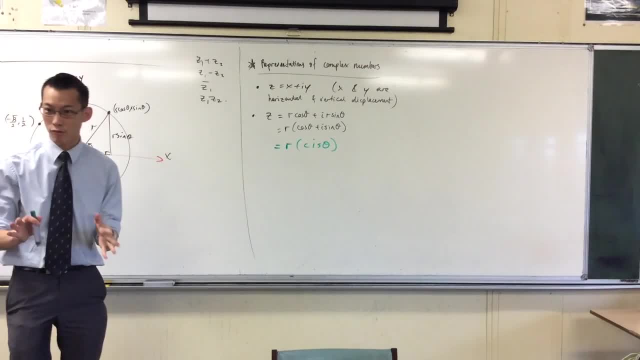 And this is pronounced r cis theta. Now I said right from the outset I'm not a huge fan of this. I don't like this as a way of notation because I mean, okay, what's good about it? It's fast. 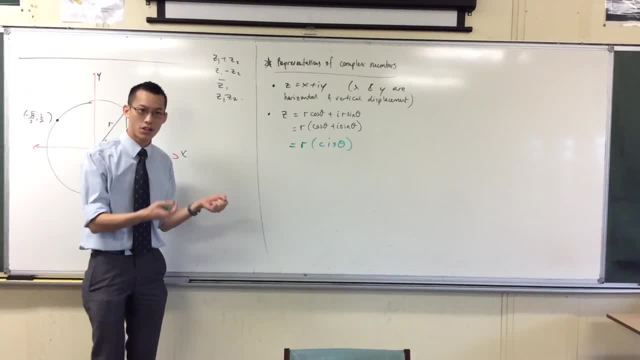 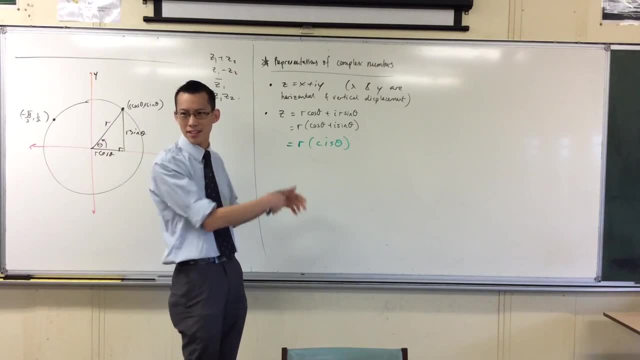 It's fast And that's about it, right. What happens is you lose. what's going on? Where does this come from? It starts to get more towards that black box, like it's just a piece of magic in its notation. I don't know what it means, but it just does its thing, okay. 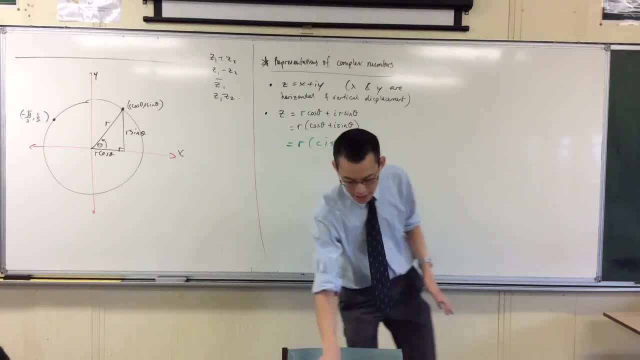 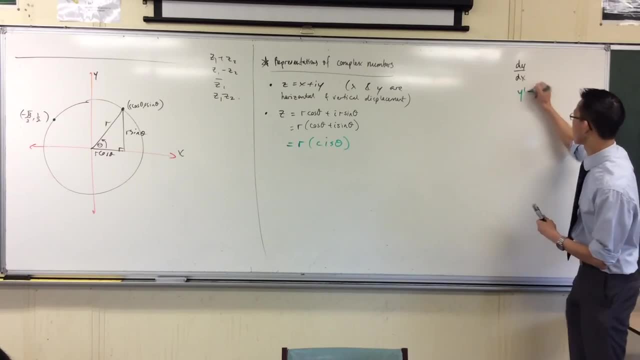 I don't like notation like that. okay, It's for the same reason, the exact same reason, that I prefer saying this as opposed to this. okay, And they're both fine And I will use both of them and you'll definitely see both of them. so you need to recognize. 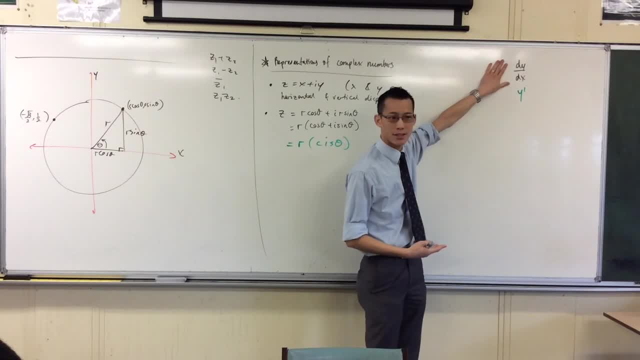 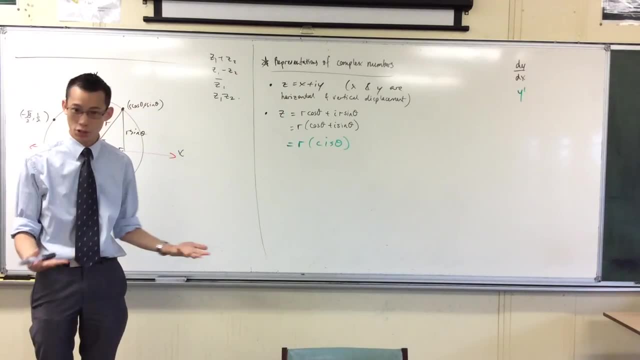 them okay, But do you see how much more meaningful this is right? It's like: why is it function? I'm doing something to it. I can see the relationship between that and rise over run, which is gradient, okay. 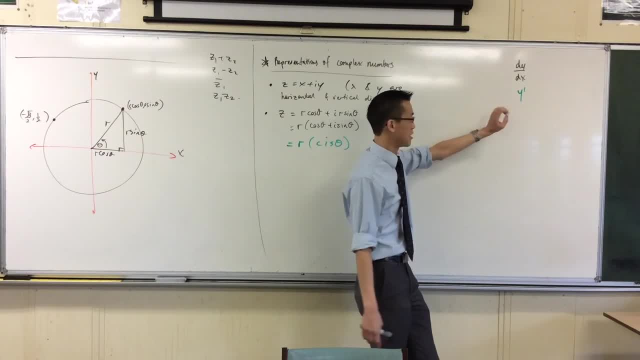 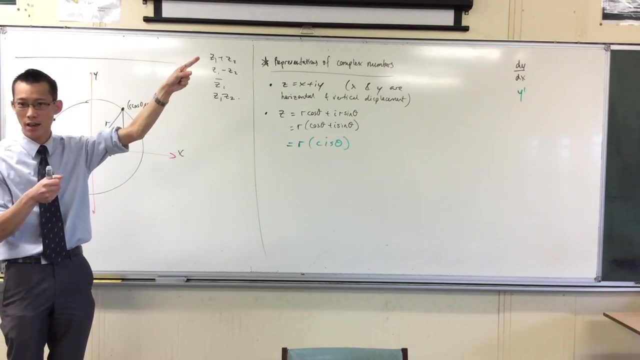 Whereas this it's like: oh, there's just some magical process And when you do it you just get a dash on there and then this is a new thing, okay, No, It's instrumentally connected to the previous thing through this mechanism of gradient. 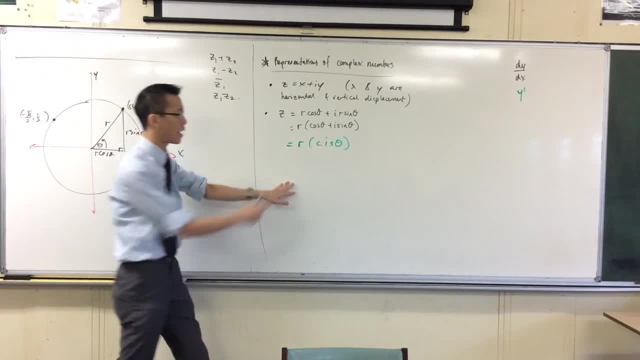 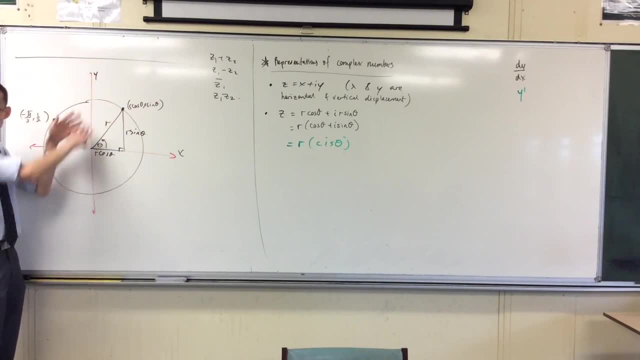 right, And the same way here. I will make a habit. I'm going to keep writing it like this, okay, Because I think it demonstrates for you what's going on here. This is what's going on. This is what's hiding underneath this notation. okay. 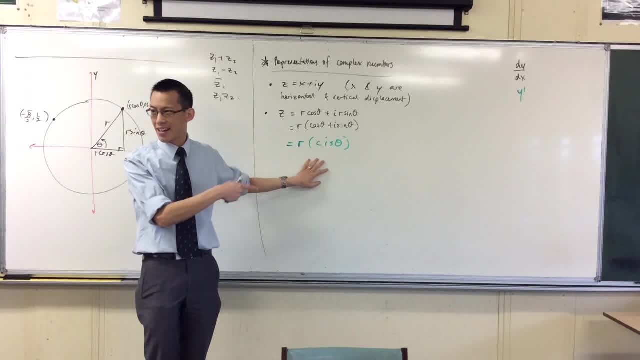 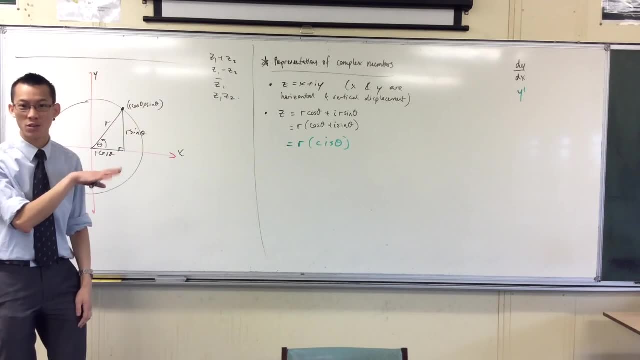 And this kind of clouds it right, But still you need to recognize it because textbooks will use it And all it means is this: Okay, so you don't need to necessarily get in a fit, but that's why I'm not using it. 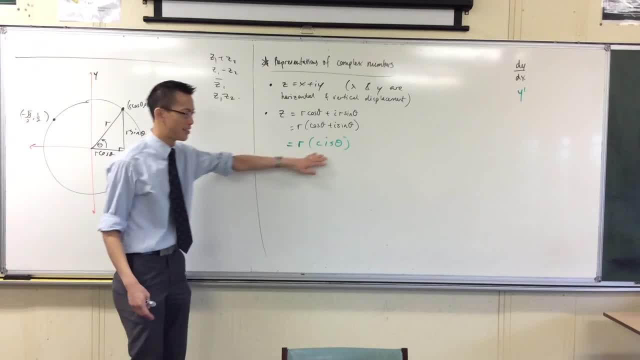 even though many other places will. And if you want to say cis-theater, then go for your life, okay, But I'm not going to.